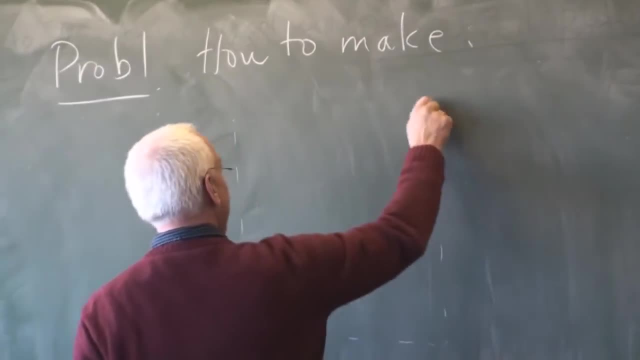 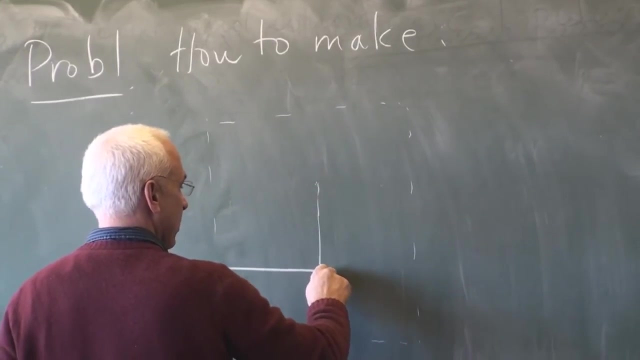 Okay so this might be a little bit challenging. So there's roughly, It's got something like that. Okay so there's a sort of a piece that goes up like this, And then there's this, This fold. Maybe the fold will be like that. 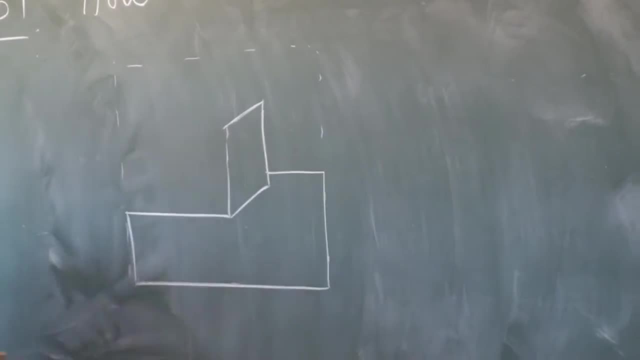 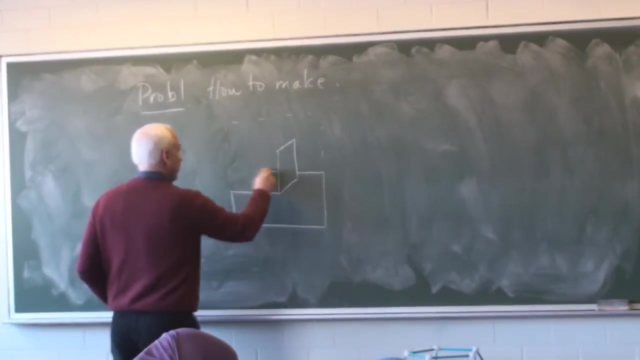 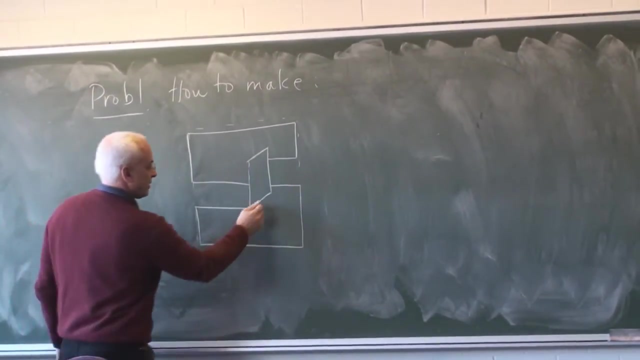 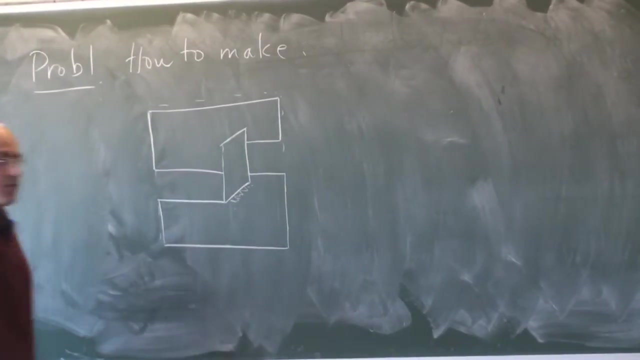 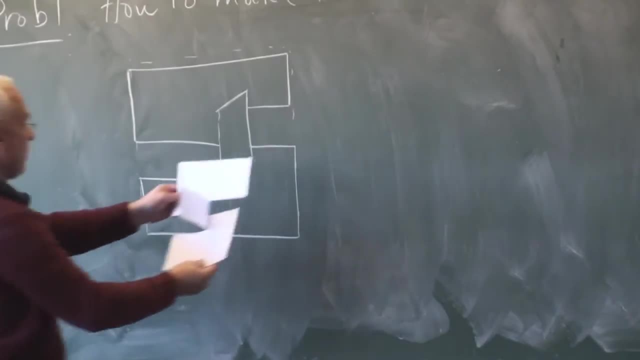 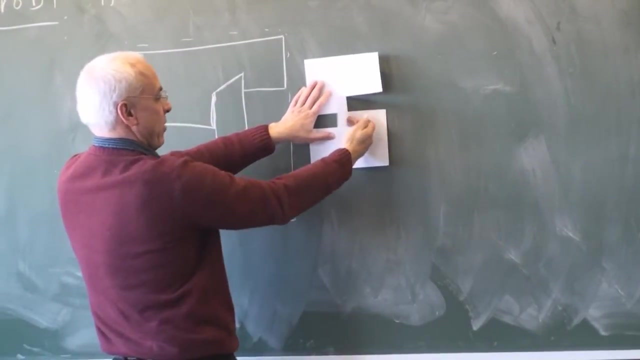 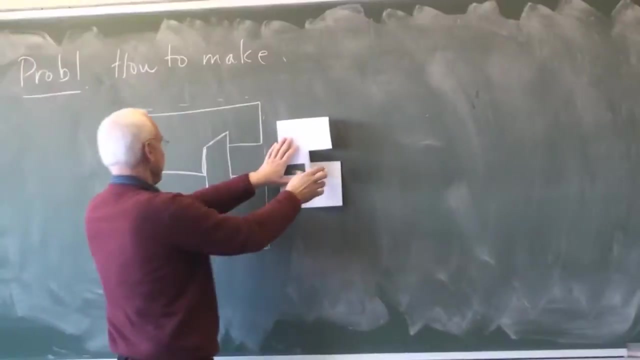 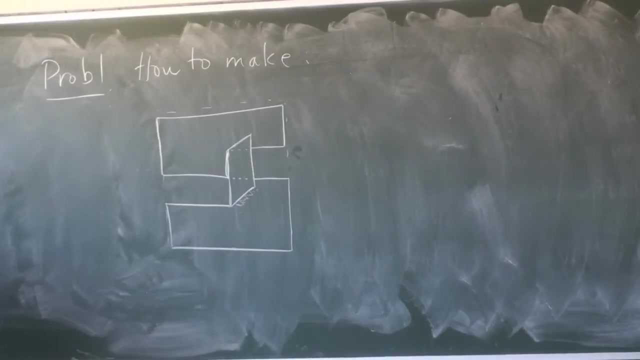 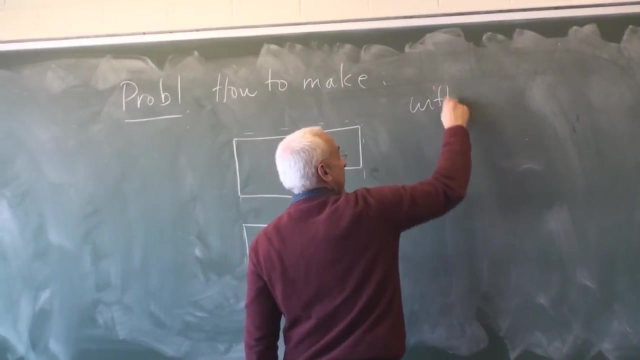 look like it. yeah, okay, so there's a fold here and there's a kind of a fold on on this side, so that that part comes up to that fold and that part comes up to that fold. so, okay, behind here this, there's something: how to make this with a single. 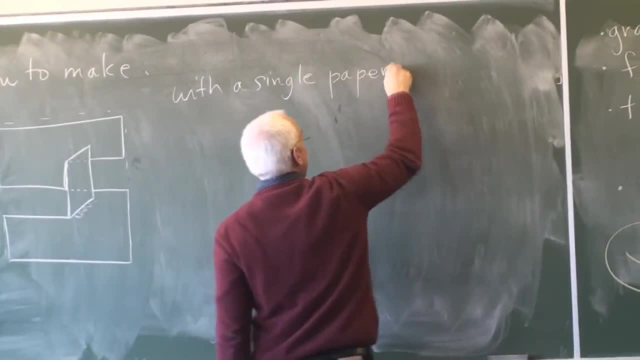 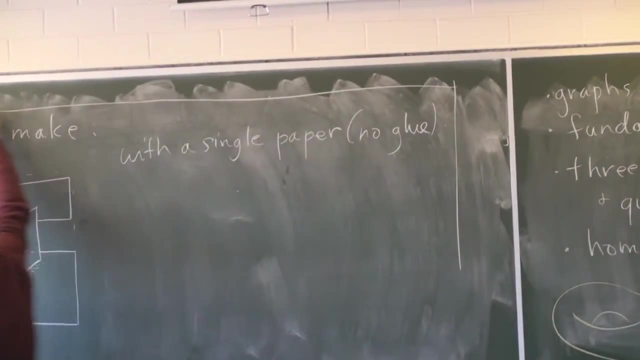 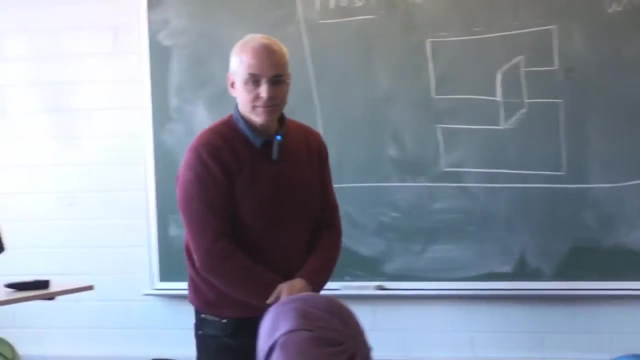 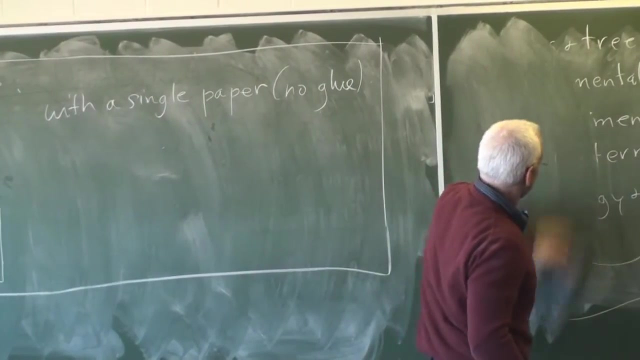 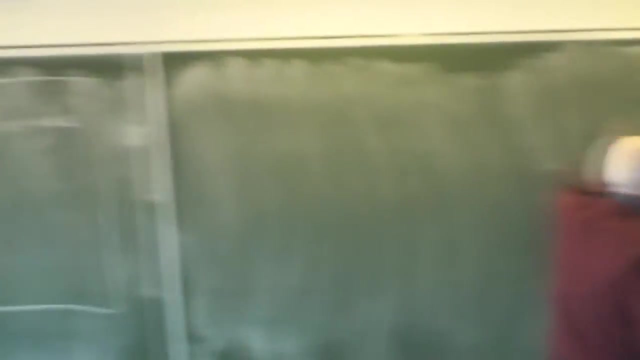 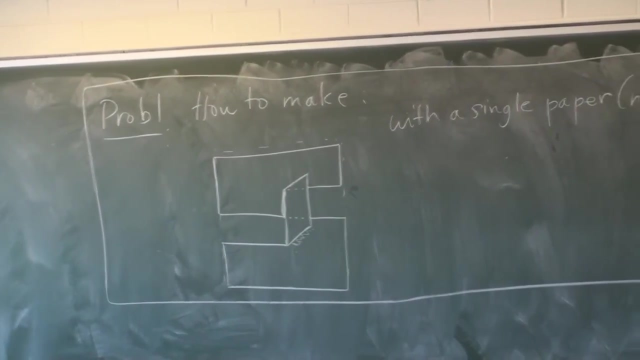 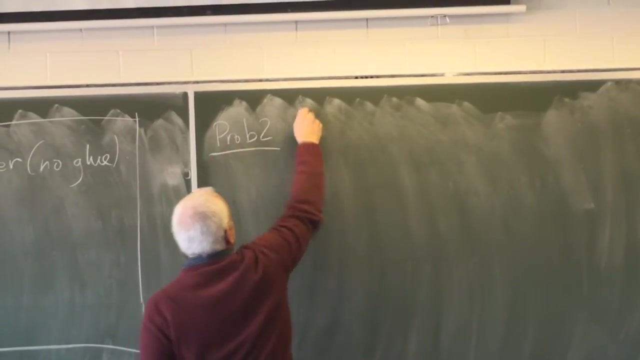 paper and no glue, all right. so there's, there's problem number one, and here's problem number two, and here's problem number two and here's problem number two. okay, this, this goes back to the famous. okay, this, this goes back to the famous. okay, this, this goes back to the famous. uh. 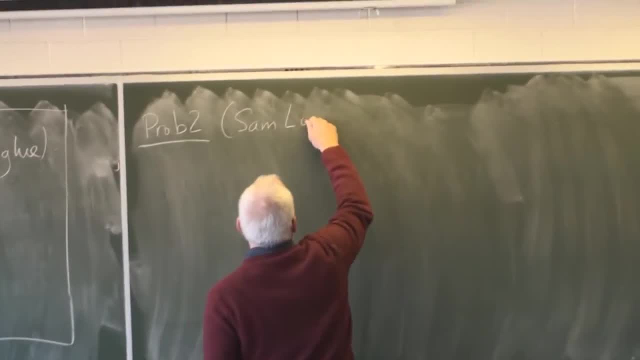 uh, uh. 19th century, 19th century, 19th century. puzzle maker named sam lloyd, puzzle maker named sam lloyd, puzzle maker named sam lloyd, who also created lots of chess, who also created lots of chess, who also created lots of chess puzzles and other things. so what you do? 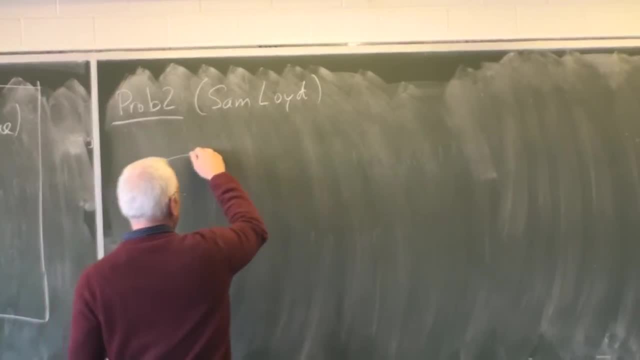 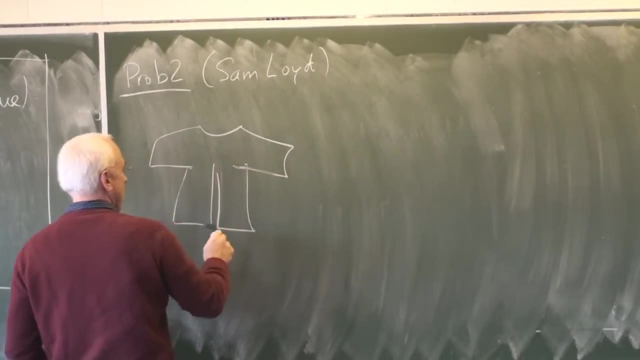 puzzles and other things. so what you do- puzzles and other things. so what you do- is you have the ingredients. are you need? is you have the ingredients? are you need? is you have the ingredients? are you need a shirt with lots of, with lots of, with lots of buttons and holes for the buttons? 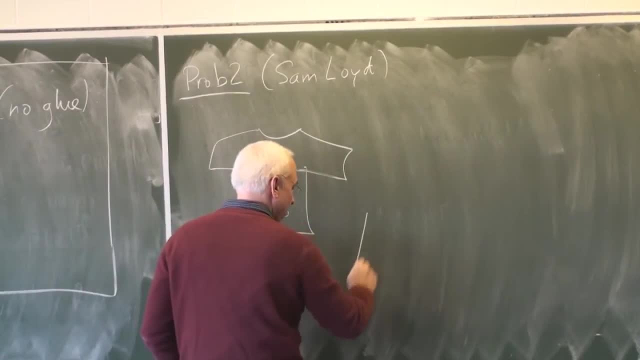 buttons and holes for the buttons. buttons and holes for the buttons. okay, and you also need a pencil. okay, and you also need a pencil. okay, and you also need a pencil. well, it doesn't have to be that big, but well, it doesn't have to be that big, but. 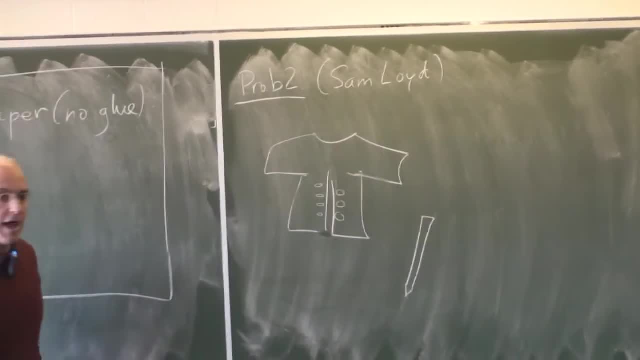 well, it doesn't have to be that big, but okay, it's a large enlarged view. there's, okay, it's a large enlarged view. there's okay, it's a large enlarged view. there's a pencil, a pencil, a pencil, and from the pencil you have a loop. 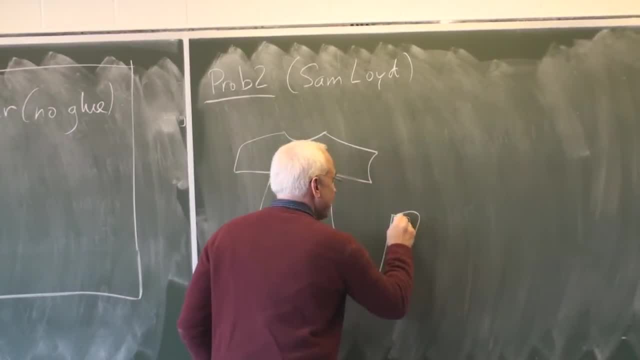 and from the pencil you have a loop, and from the pencil you have a loop, you've got a piece of string. you've got a piece of string. you've got a piece of string which is looped like this: so this is a which is looped like this. so this is a. 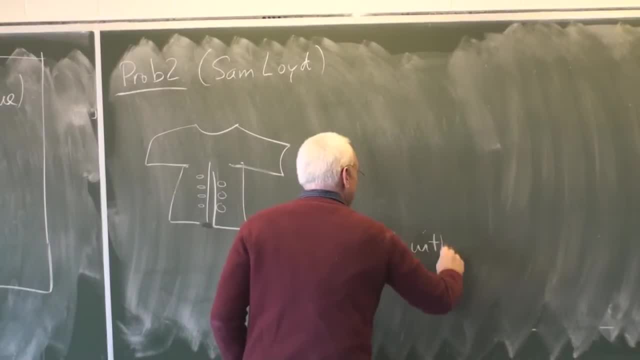 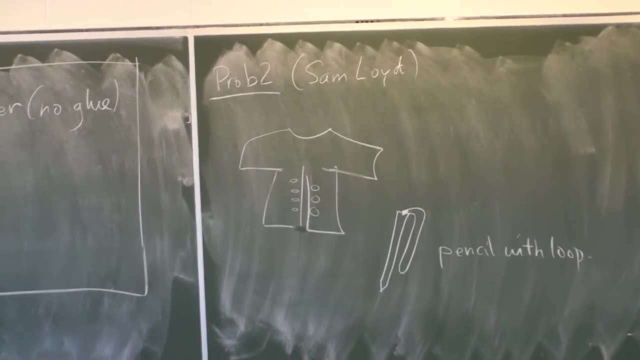 which is looped like this. so this is a pencil, pencil with a loop, with a loop, with a loop, and the loop is, and the loop is, and the loop is not big enough to go over the pencil, not big enough to go over the pencil, not big enough to go over the pencil. okay, even if you pull it tight, it's not. 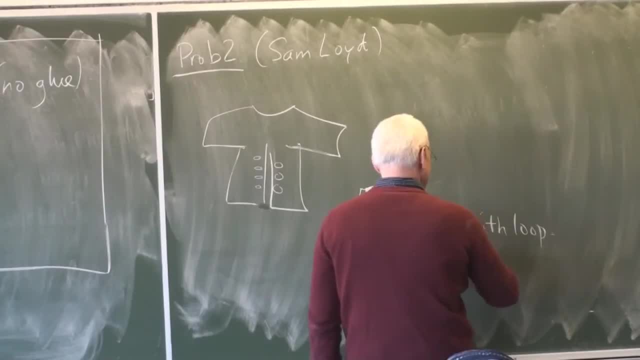 okay, even if you pull it tight, it's not okay. even if you pull it tight, it's not big enough to go over the pencil, big enough to go over the pencil, big enough to go over the pencil. so, with a loop which is a smaller, so with a loop which is a smaller. 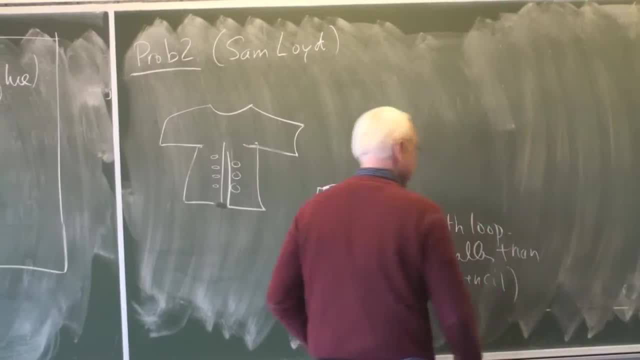 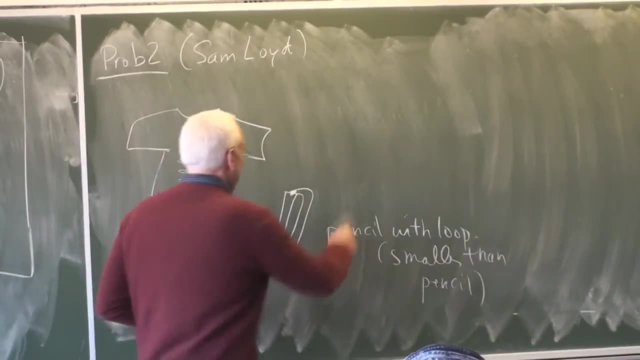 so with a loop which is a smaller than the pencil, okay, and so these are the ingredients. okay, and so these are the ingredients. okay, and so these are the ingredients. and then what we do is, and then what we do is, and then what we do is: if you know how to do it, what you do is: 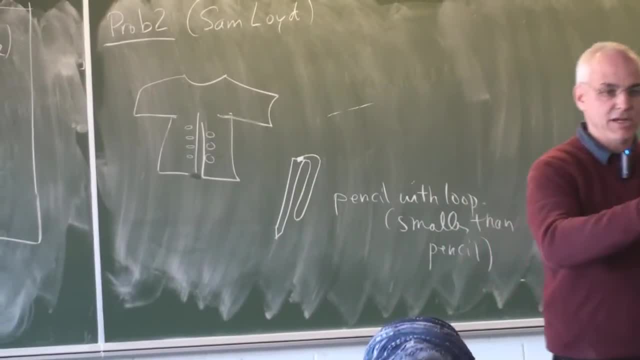 if you know how to do it, what you do is: if you know how to do it, what you do is: you take the shirt and you can actually. you take the shirt and you can actually. you take the shirt and you can actually do it on with somebody's shirt if you. do it on with somebody's shirt. if you do it on with somebody's shirt, if you have one of these things, you can do it. have one of these things, you can do it. have one of these things, you can do it. you say: what look the other way for a. 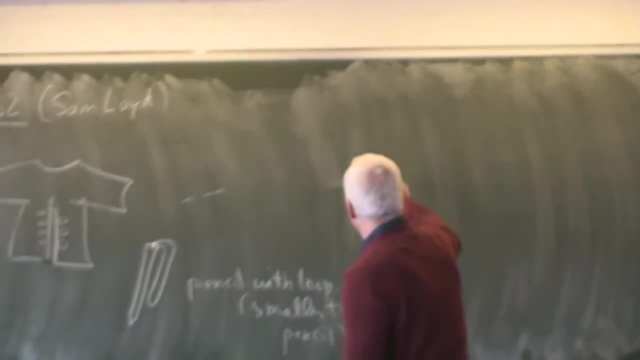 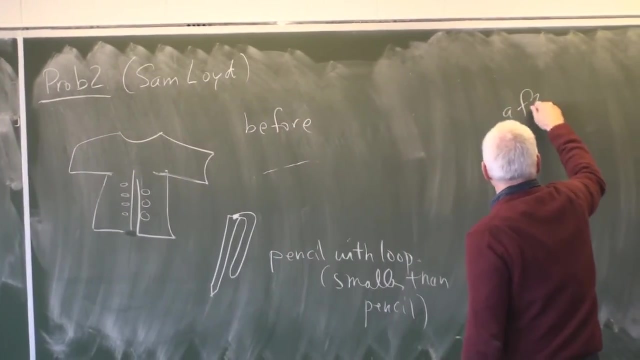 you say: what look the other way for a, you say what look the other way for a second, and you do something quickly and second, and you do something quickly and second, and you do something quickly. and then then, then afterwards- this is before and then after- you end up with something that looks. 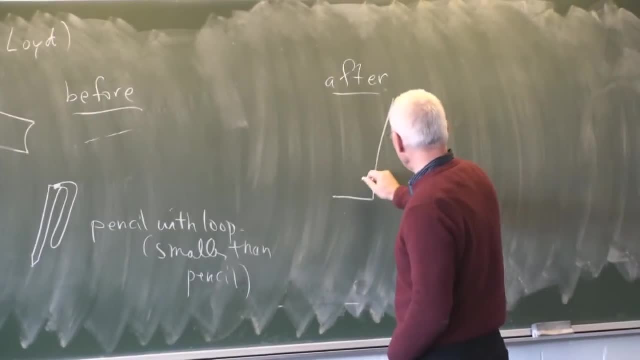 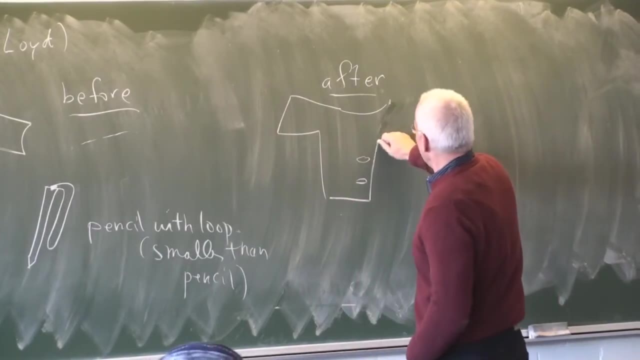 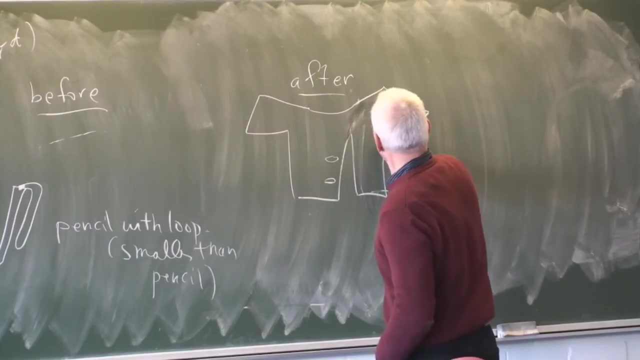 you end up with something that looks. you end up with something that looks like this, like this, like this: okay, um, okay, so here's our our shirt, the buttons there. okay, so we've taken the buttons there. okay, so, we've taken the buttons there. okay, so we've taken one of the holes. 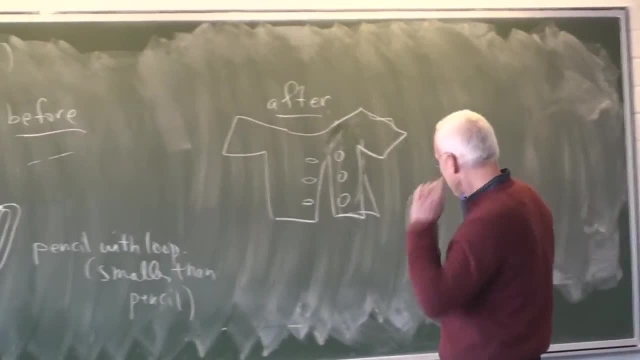 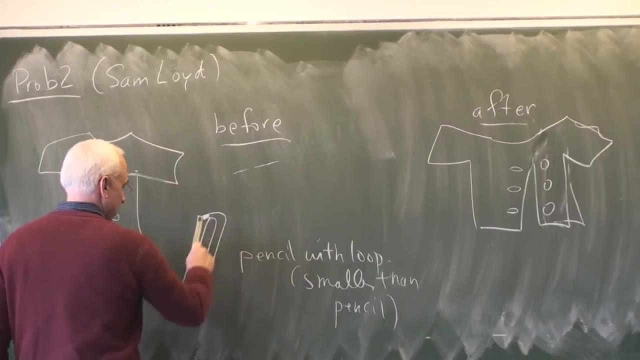 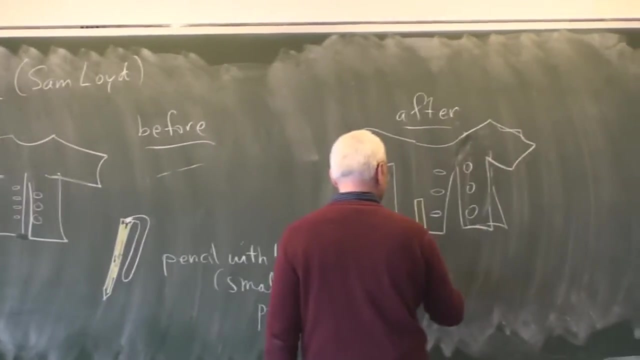 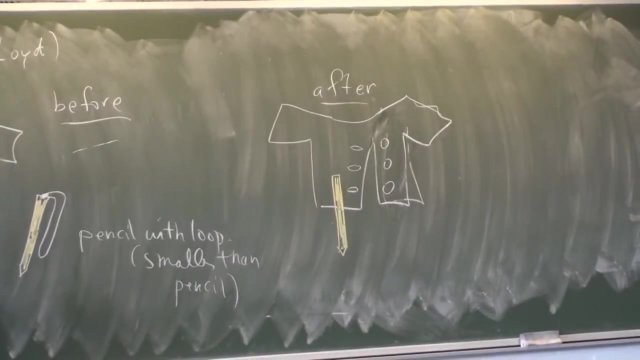 one of the holes, one of the holes, and what happens? and what happens, and what happens. i'll call this pencil yellow. i'll call this pencil yellow. i'll call this pencil yellow. okay, so the pencil is now like this: and uh, what about the? and uh, what about the? 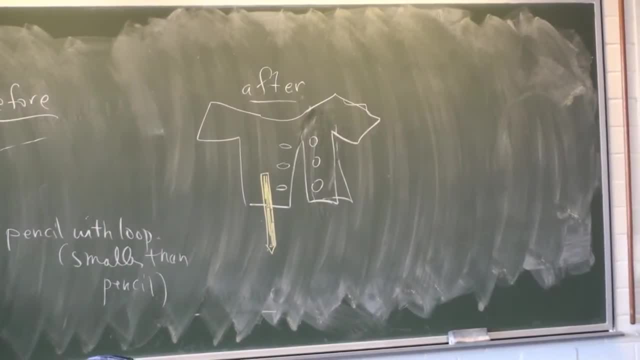 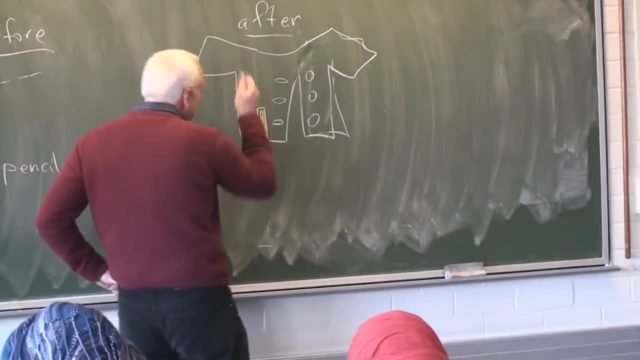 and uh, what about the the loop? well, maybe it'll be purple- there's our well. maybe it'll be purple- there's our. well, maybe it'll be purple- there's our purple loop. the loop looks like this. the loop looks like this. the loop looks like this: now it goes through here. 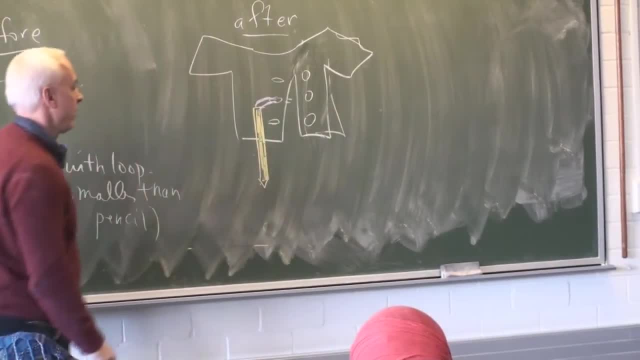 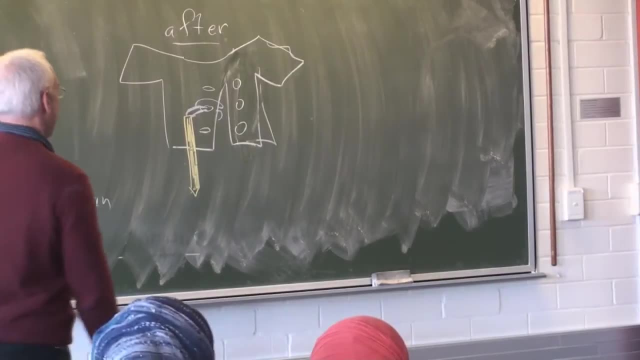 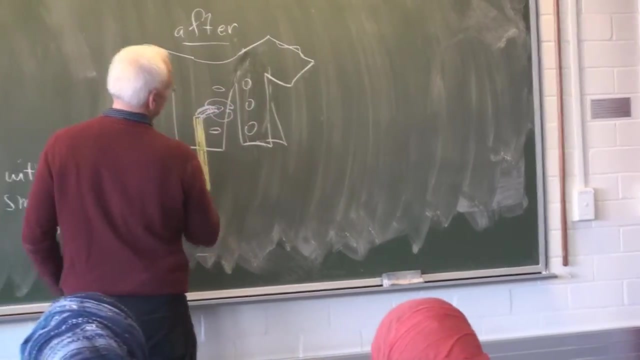 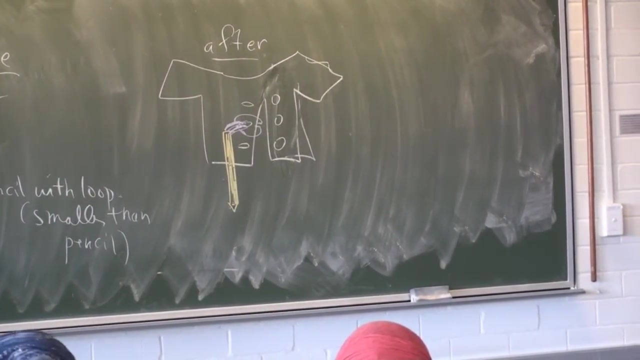 now it goes through here. now it goes through here. then it comes out the back and goes under, goes under, goes under. so it only uses one hole of the shirt. so it only uses one hole of the shirt. so it only uses one hole of the shirt. yeah, just uses one hole of the shirt. 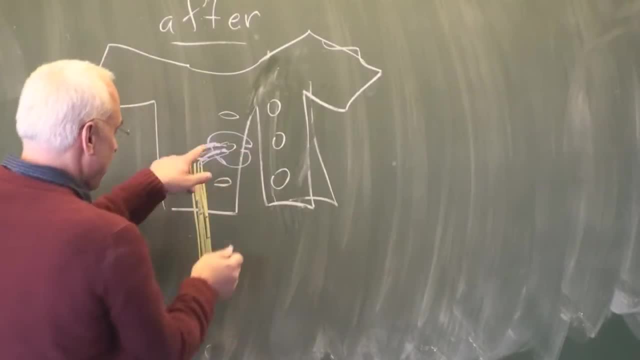 yeah, just uses one hole of the shirt. yeah, just uses one hole of the shirt. okay, so, um, so, so. the pencil is now okay. so, um, so, so. the pencil is now okay. so, um, so, so. the pencil is now attached to the shirt. but attached to the shirt, but. 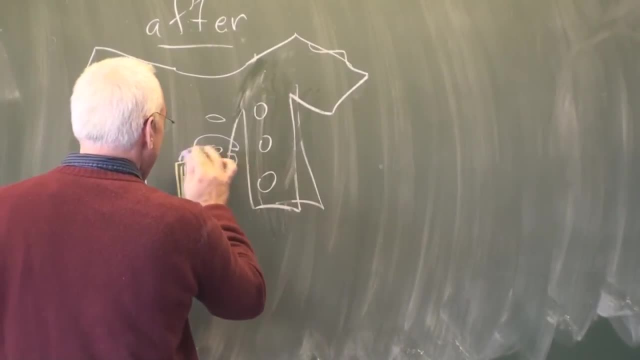 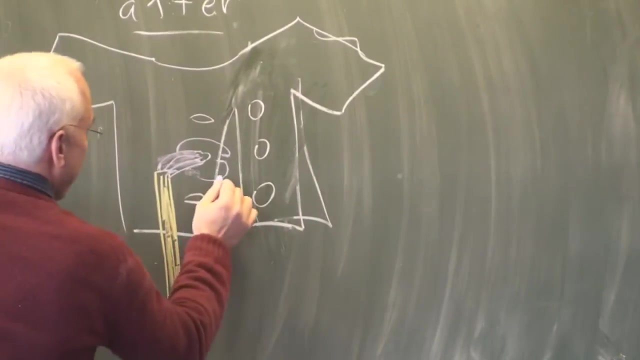 attached to the shirt, but this part goes over. let me try to make this part goes over. let me try to make this part goes over. let me try to make that a little bit more clear. so there's that there. so there's that there. so there's that there that goes into the hole and then. 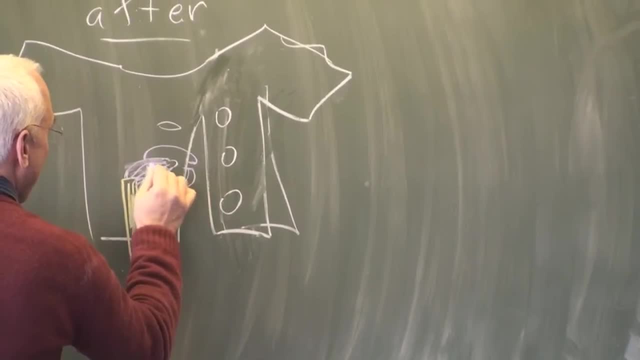 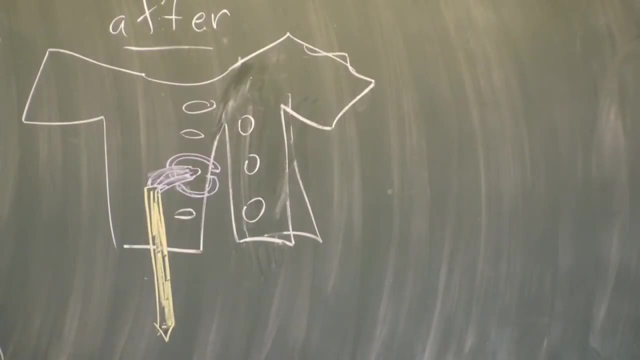 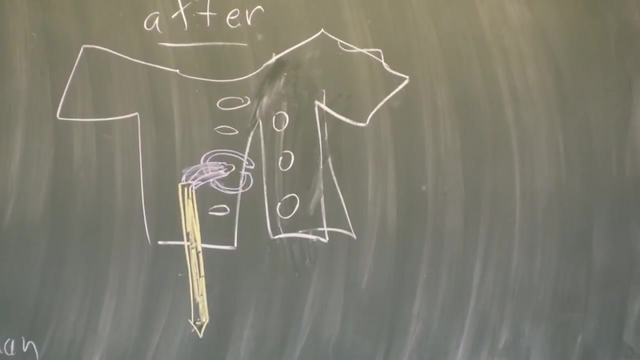 that goes into the hole, and then that goes into the hole and then outside here, oh yeah, we need to preserve holes. this, oh yeah, we need to preserve holes. this, oh yeah, we need to preserve holes. this is a topology, is a topology, is a topology. this is a solid piece of string. this is a. 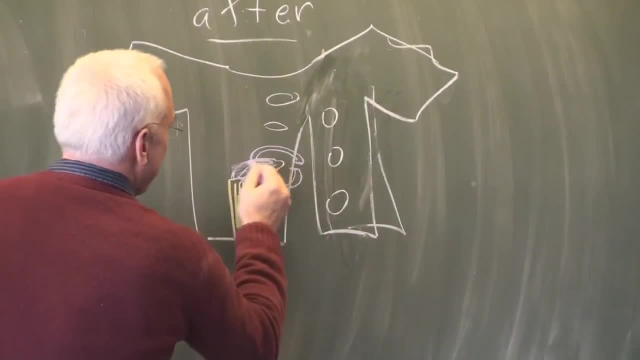 this is a solid piece of string. this is a. this is a solid piece of string. this is a solid piece of string. solid piece of string. this is a solid piece of string. solid piece of string. this is a solid piece of string. okay, okay, i'll draw it. okay, okay, i'll draw it. okay. okay, i'll draw it. i'll just make it a little bit thicker. i, i'll just make it a little bit thicker. i, i'll just make it a little bit thicker. i want to make it clear that this is in. 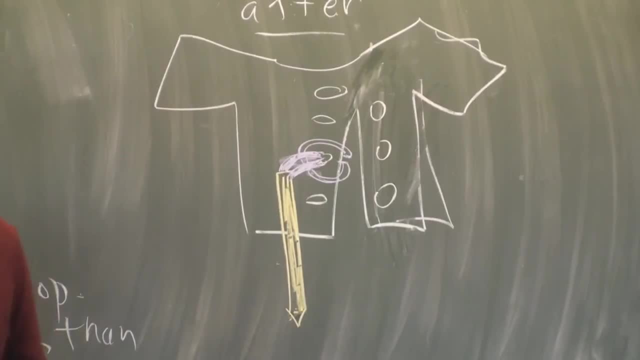 want to make it clear that this is in, want to make it clear that this is in front and that's behind front, and that's behind front and that's behind. so, so, so, so, it's all so the thing. so, so, so, so, it's all so the thing.